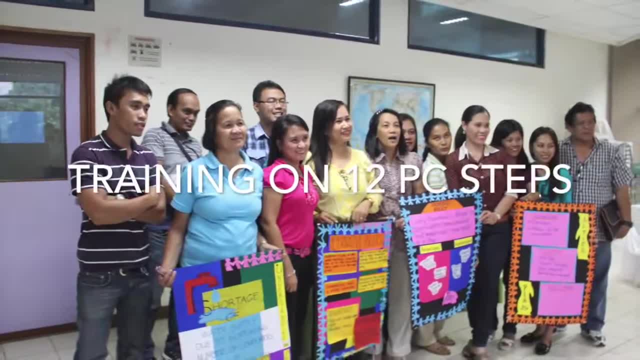 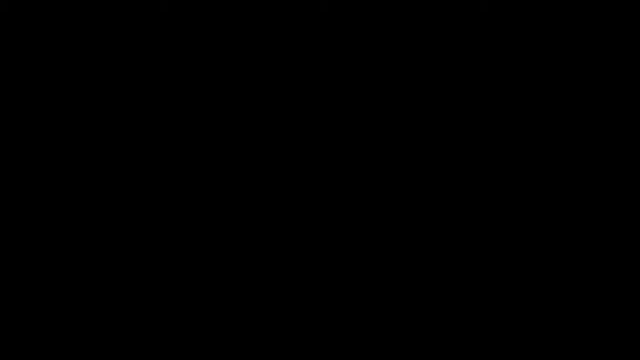 Project Citizen: the creation of themes and training on the 12 steps of Project Citizen, where the end goal is for the teachers to learn how to be the moderators themselves. 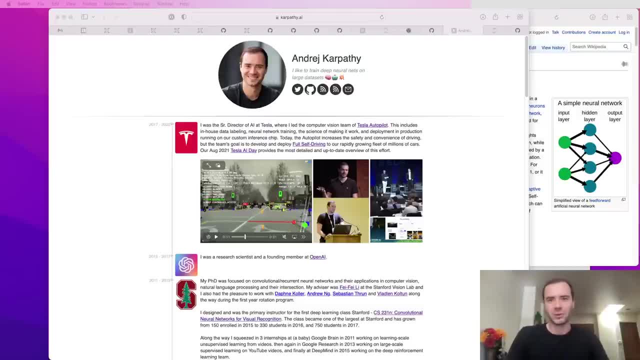 Hello, my name is Andre and I've been training deep neural networks for a bit more than a decade, And in this lecture, I'd like to show you what neural network training looks like under the hood. So, in particular, we are going to start with a blank Jupyter notebook and by the end of this, 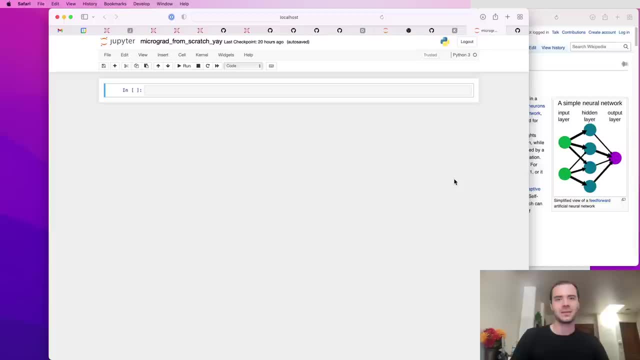 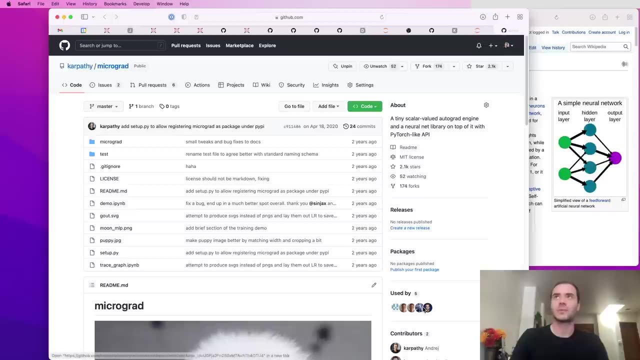 lecture, we will define and train a neural net and you'll get to see everything that goes on under the hood and exactly sort of how that works on an intuitive level. Now, specifically, what I would like to do is I would like to take you through building of micrograd, Now micrograd. 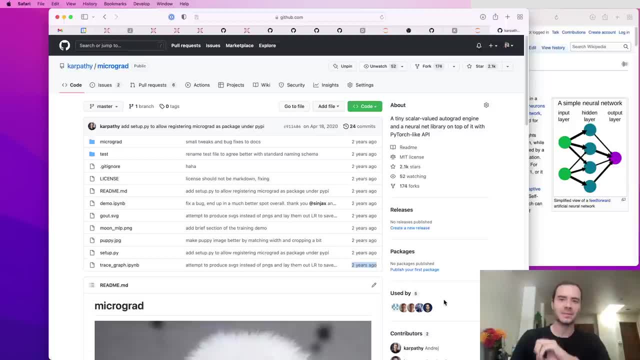 is this library that I released on GitHub about two years ago, but at the time I only uploaded the source code and you'd have to go in by yourself and really figure out how it works. So in this lecture I will take you through it step by step and kind of comment on all the pieces of it. 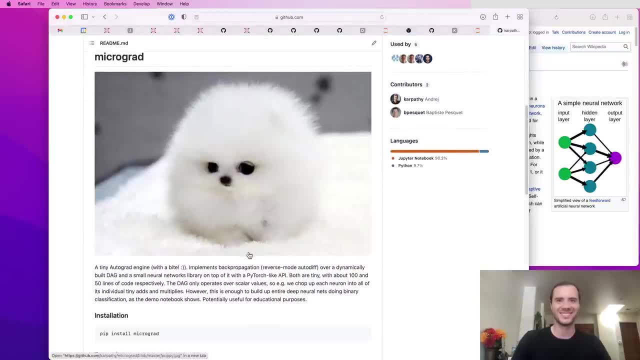 So what's micrograd and why is it interesting? Thank you. Micrograd is basically an autograd engine- Autograd is short for automatic gradient- and really what it does is it implements back propagation. Now, back propagation is this algorithm that allows you to efficiently evaluate the gradient of some kind of a loss function with. 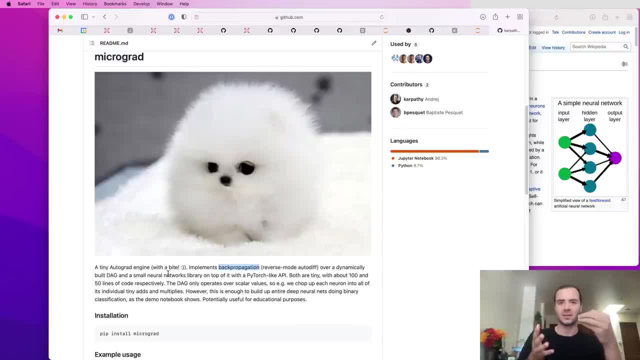 respect to the weights of a neural network, and what that allows us to do, then, is we can iteratively tune the weights of that neural network to minimize the loss function and therefore improve the accuracy of the network. So back propagation would be at the mathematical core of any modern deep neural network library, like, say, PyTorch or JAX. So the functionality 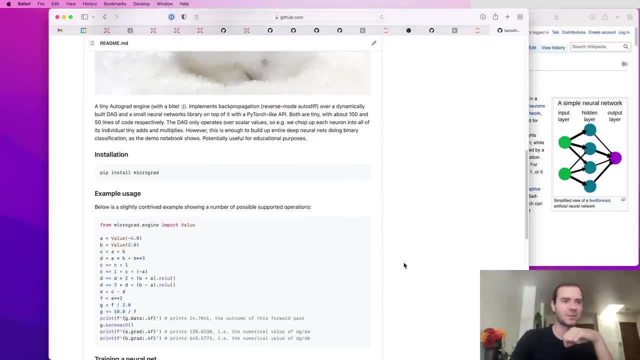 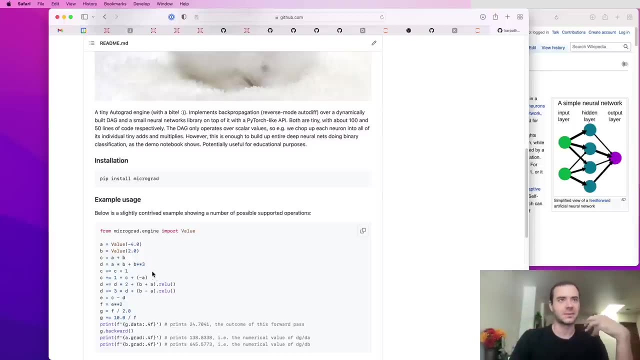 of micrograd is, I think, best illustrated by an example. So if we just scroll down here, you'll see that micrograd basically allows you to build out mathematical expressions, and here what we are doing is we have an expression that we're building out, where you